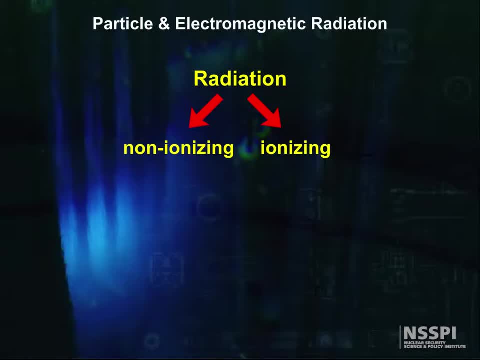 While non-ionizing radiation can certainly be dangerous, consider microwaves, for example. for this course, we will focus exclusively on ionizing radiation. So the first rhetorical question: what do we mean by ionizing radiation? That goes all the way back to what do we mean by an ion, If you remember from your physics and chemistry. 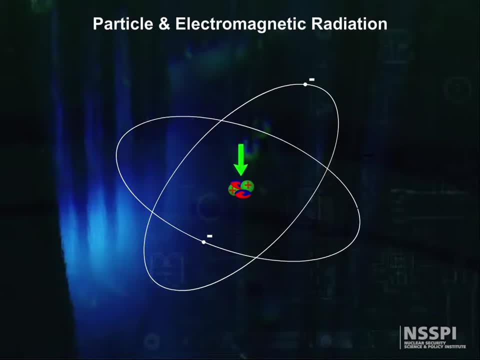 neutral atoms contain two fundamental parts: The nucleus, which is very small, very heavy and contains one or more positive charges, and the surrounding cloud of electrons that contain the same number of of negative charges. When one of these electrons is removed from the neutral 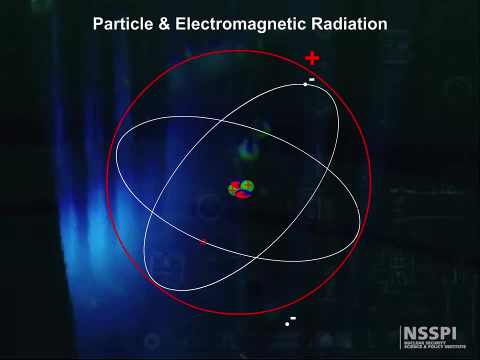 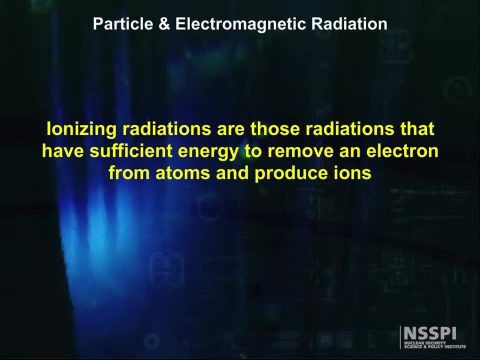 atom. the remaining atom that's missing- electrons- is called an ion. Ionizing radiation is thus defined as those radiations that have sufficient energy to remove electrons from atoms and produce ions. What's so special about ions? This is a far deeper question than you might realize, Although ions are very 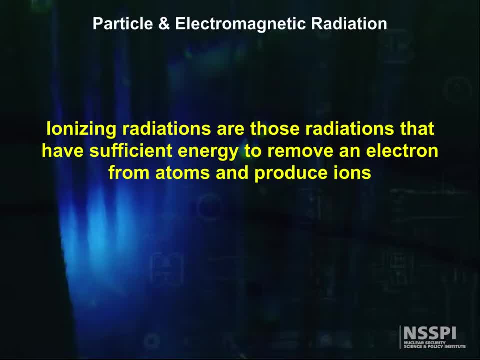 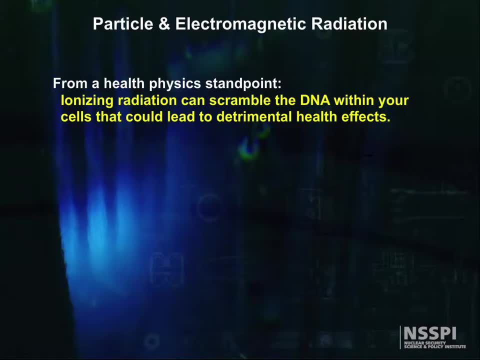 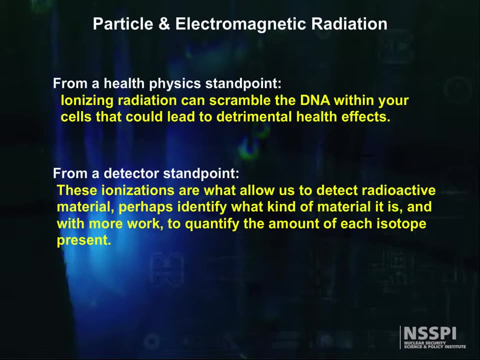 common. those from radiation are particularly important to us. From a health physics standpoint, ionizing radiation can scramble the DNA within your cells and could lead to detrimental health effects. From the detector standpoint, it is these ionizations that allow us to detect radioactive material. 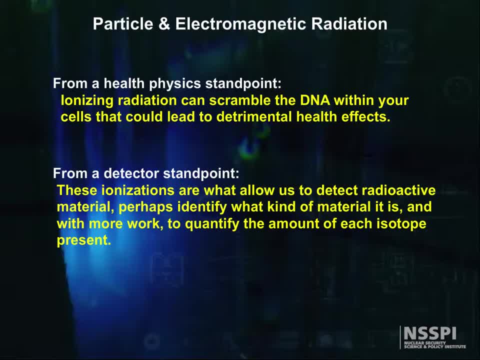 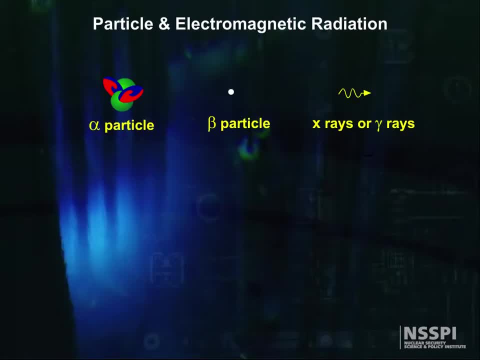 perhaps identify what kind of material it is And, with more work, to quantify the amount of each isotope present, challenging. On a historical note, the scientists who discovered radiation in the early days were not particularly inventive. Alpha, beta and gamma were the first three. 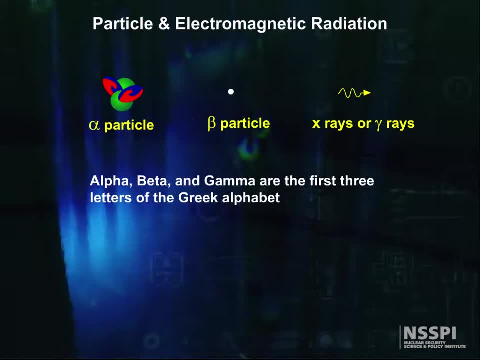 letters of the greek alphabet, And x-rays were so named because Röntgen didn't know what they were, So he named them X for the unknown. An alpha particle is a helium nucleus ejected from a Mercury watching at random another galaxy. 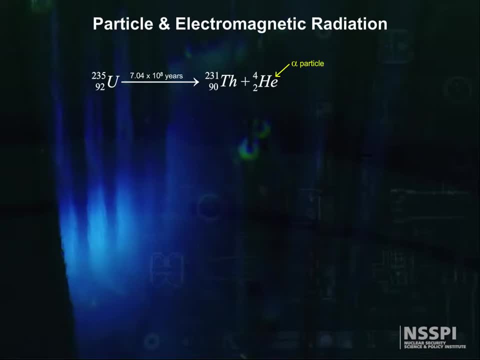 directly from the parent or decaying nucleus. A typical alpha decay is the following: U-235 decays to Thorium-231 plus an alpha particle with a half-life of 7.038 times 10 to the 8th years. Let's talk for a minute about what. 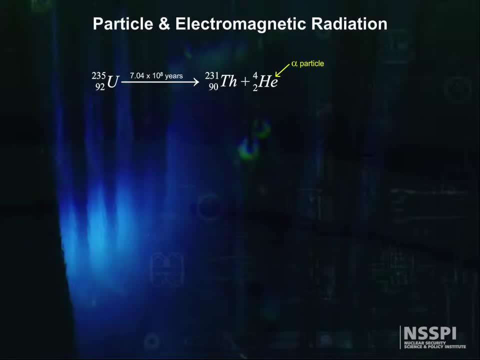 everything means in these equations and what the rules are. The 92 sitting next to the symbol for uranium is the charge of the nucleus. In this case it's the atomic number: 92 protons. The 235 is the mass number, that is, the total number of. 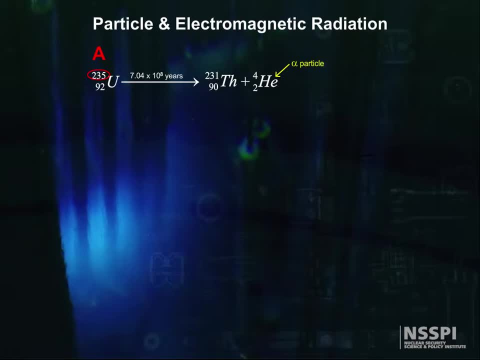 nucleons in the uranium nucleus, In this case 92 protons and 143 neutrons. Likewise for Thorium that has an atomic number of 90, and helium with an atomic number of 2.. If you think about it, the sum of the mass numbers on the 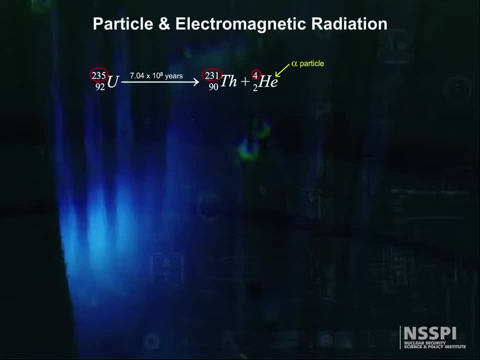 right-hand side of the equation must equal to the mass number on the left-hand side of the equation. Also, one of the deep conservation laws of the universe is that charge is always conserved. So for this equation 92 is equal to 90 plus 2.. The half-life for alpha decay for uranium-235 is about: 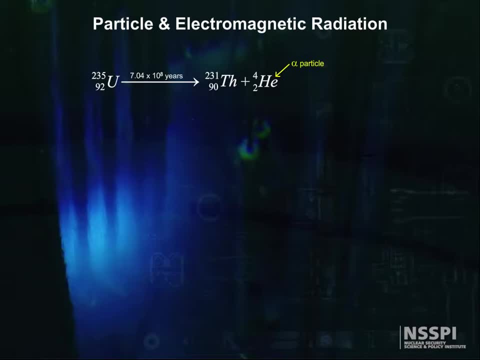 704 million years. We've seen beta minus decay already, but now let's name the parts. Tritium, with a half-life of 12.33 years, decays to helium-3 plus an electron plus an antineutrino. 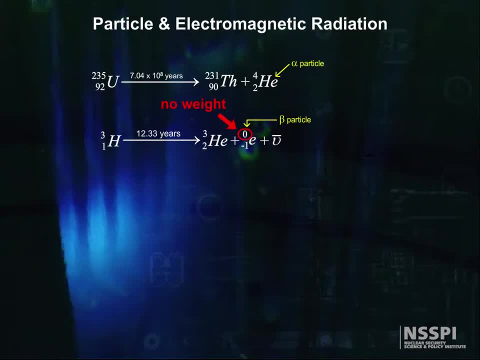 Whoa, An electron doesn't weigh anything. Yep, it's true. On the scale of nucleons, zero is good enough for electrons in these balance equations. When we go to calculate mass-energy relationships, then we have to worry about the mass of an electron, but that's for another day. 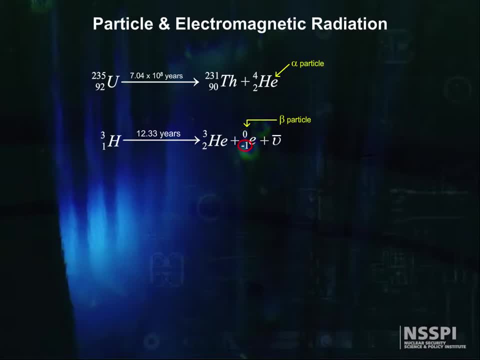 Looking at the electron again, we see that it has a minus one charge and, given that our rule about conserving charge and mass number is kept, Neutrinos, the new bar thing on the right-hand side of the equation, is for another day also, But it 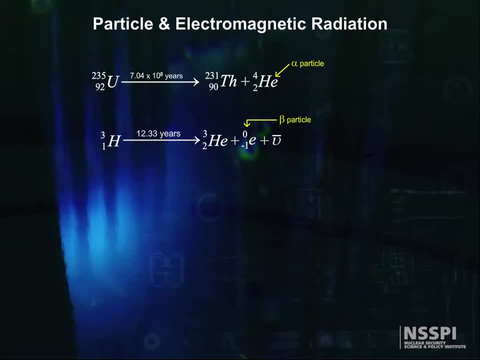 has no charge and essentially no mass, even compared to an electron, so we can gleefully ignore it for now. Suppose the nucleus has too many protons. How does it change? How does it change the proton to a neutron? By positron or beta-plus decay like